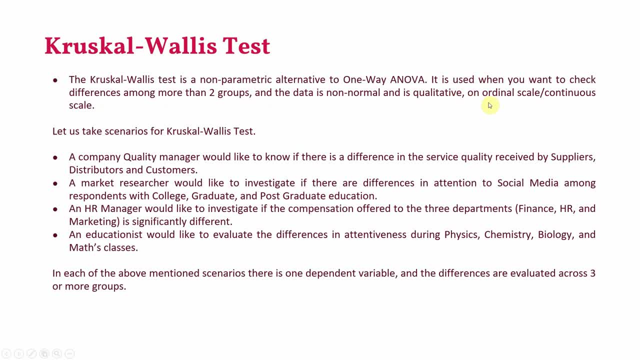 can be continuous, non-normal or qualitative on ordinal scale. Let us take scenarios for Kruskal-Wallis test. A company quality manager would like to know if there is a difference in service quality received by suppliers, distributors and customers. A market researcher would like to investigate if there are differences in attention to social. 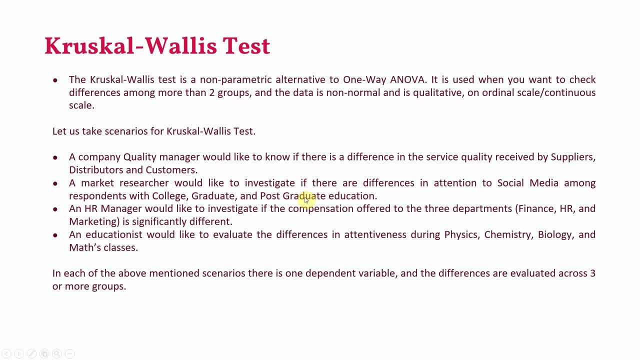 media among respondents with college, graduate and postgraduate education. An HR manager would like to investigate if the compensation offered to the three departments is significantly different. An educationist would like to evaluate the differences in attentiveness during physics, chemistry, biology and maths classes. 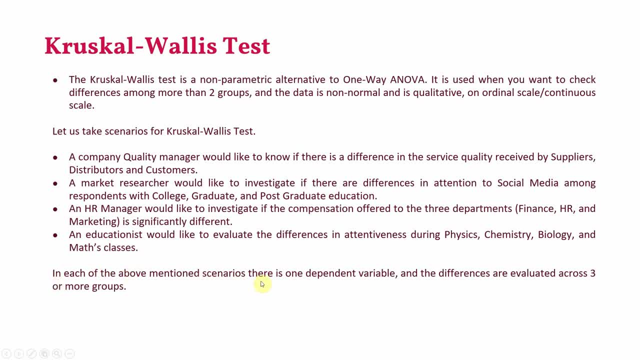 In each of the above-mentioned scenarios there is one dependent variable. In the first scenario we have service quality, In the second attention to social media, In the third compensation And in the fourth attentiveness, And the differences are evaluated across three or more groups. 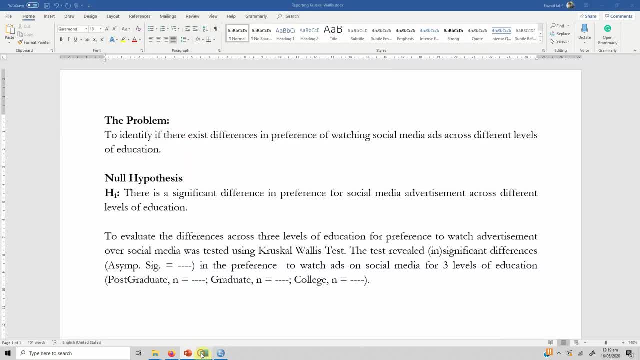 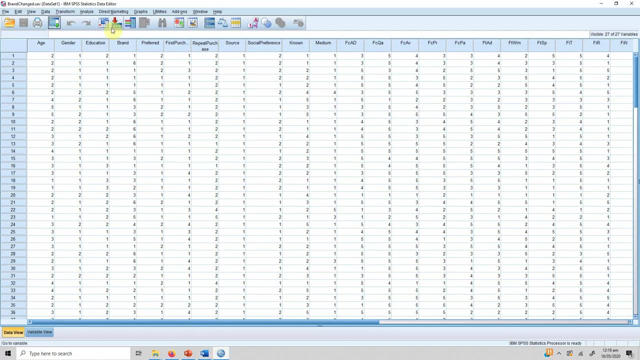 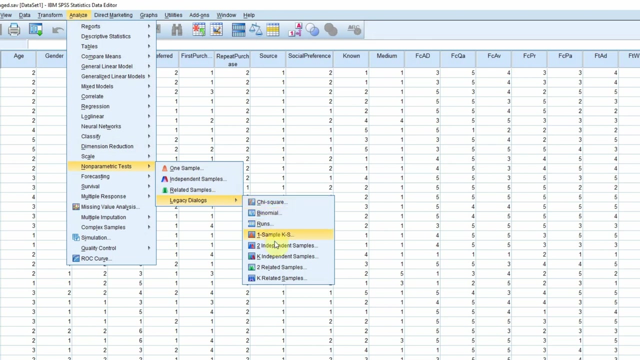 In order to run Kruskal-Wallis test, we are taking this example whereby we want to identify if there exist differences in preference of watching social media ads across different levels of education. So, how to run Kruskal-Wallis test, You will go to analyze non-parametric test, legacy dialogues and k independent samples. 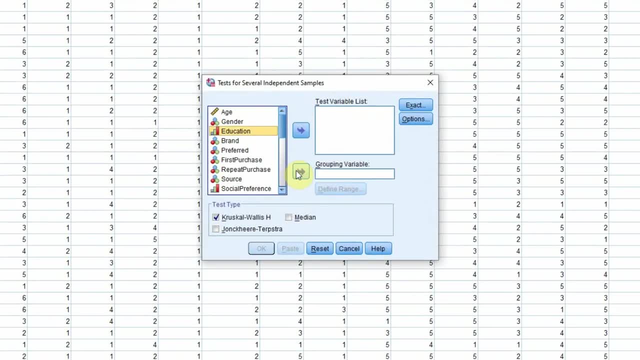 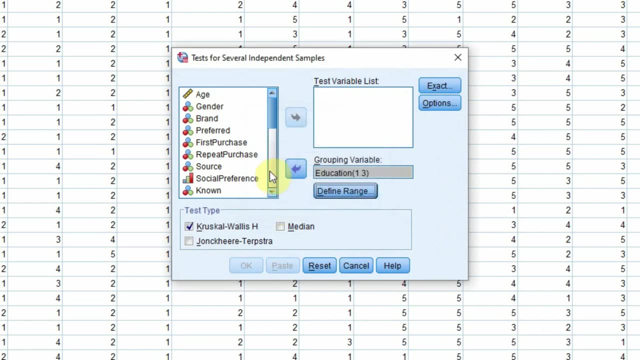 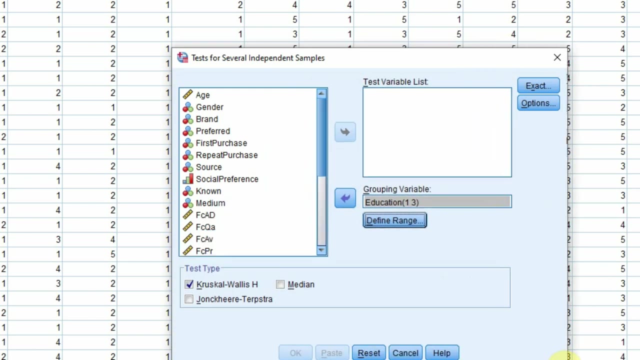 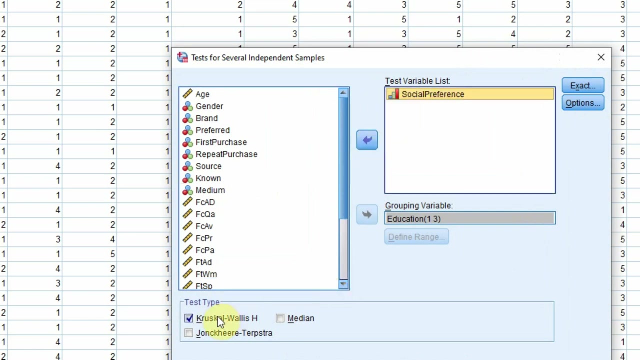 Click on it. We are interested in education as our grouping variable. So there are three groups, starting from one up until three, And we are interested in the other variable. The dependent variable is social preference. The Kruskal-Wallis H is selected. 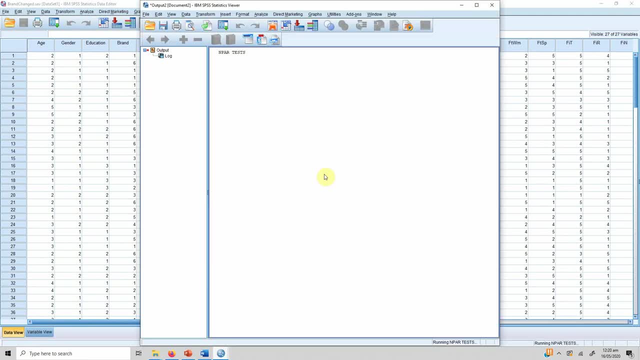 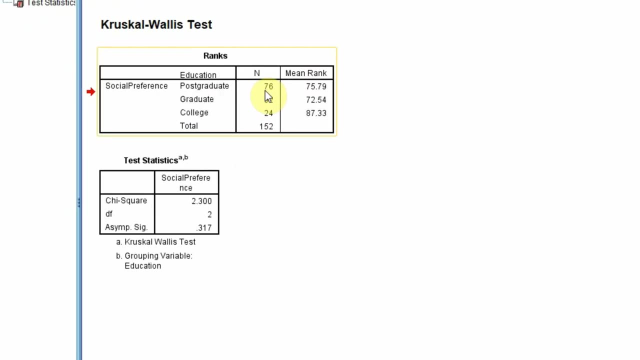 And what we do is we press OK. Now Here are our results. Now, if we have a look here, we have got 76 respondents who have got postgraduate education, 52 who have got graduate education and 24 who have got college education.